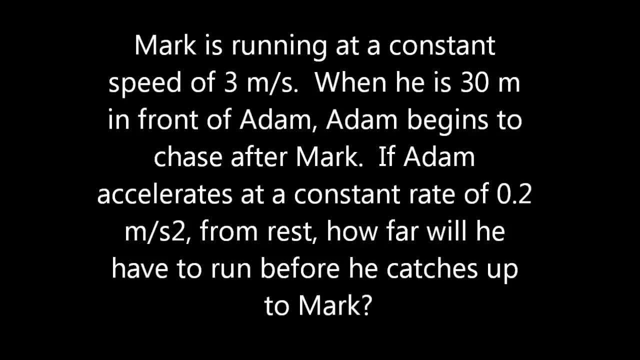 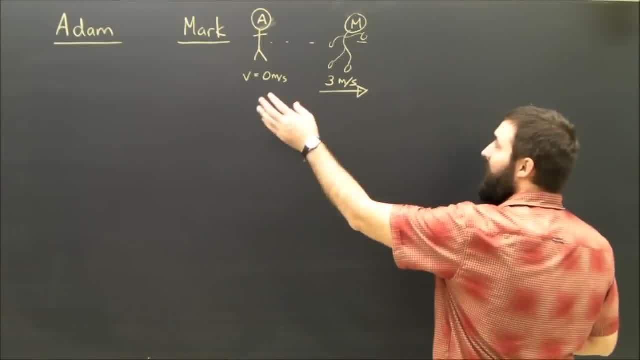 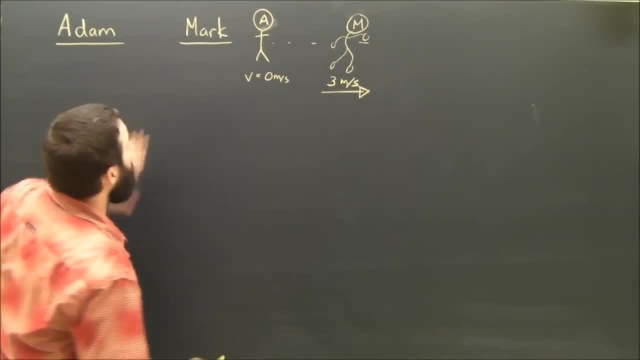 Okay, so you've read the question. We've got Adam and he's chasing Mark. Mark is running at a constant velocity of 3.. We've got two people in this question, so let's do two sets of givens For Mark. his velocity, as I just said, was 3 meters per second. He's running. 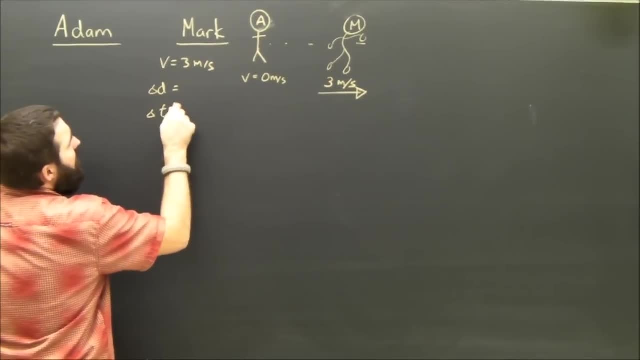 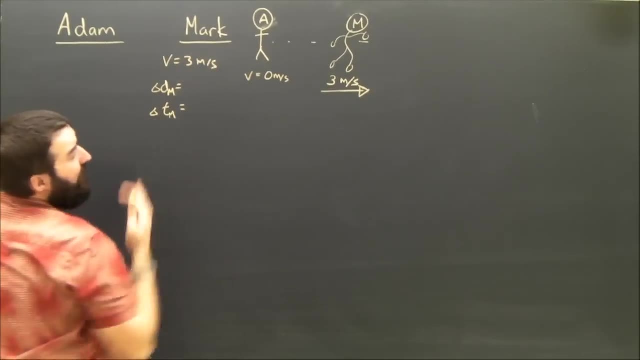 at a constant velocity, which means the only variables we need are v, d and t. I'm going to call that dm for Mark, tm the time for Mark, But the only thing I know is 3, so let's hang on one second there and let's look at Adam for a second. Adam starts from rest. 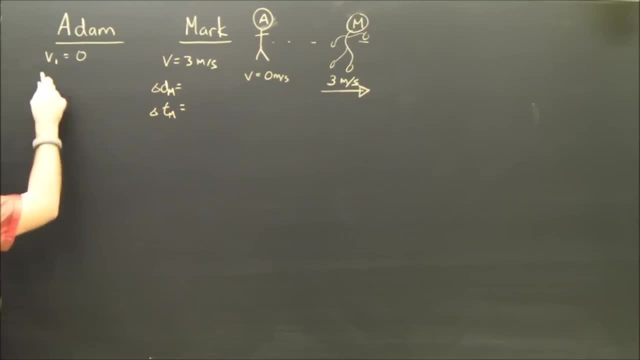 Well, that means, of course, that v1 is equal to 0. And as soon as I write v1, I'm going to have to write v2.. I'm going to write a. I'm going to write delta d. I'm going to write: 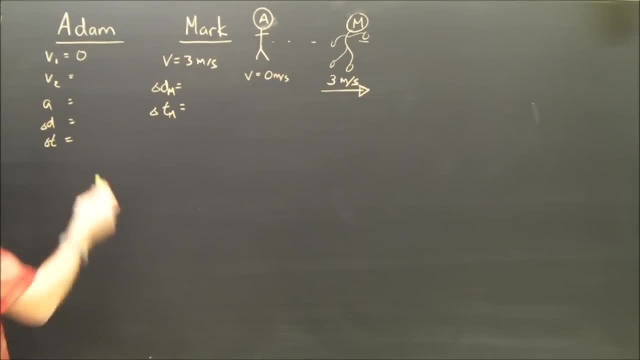 delta, t, all five of the variables that belong to my kinematics equations, the big five. So v1 for Adam is 0, and he's running at a constant velocity of 3 meters per second. He's accelerating. It's set at 0.2 meters per second squared. And here I'm going to. 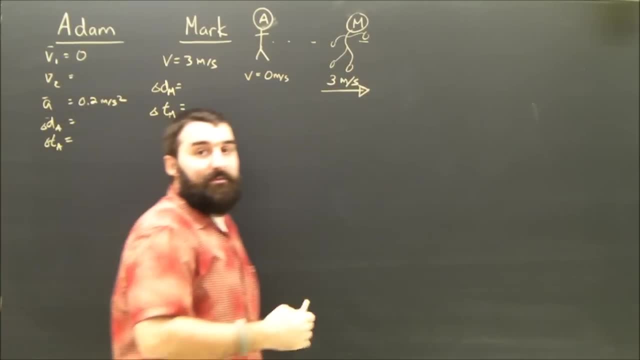 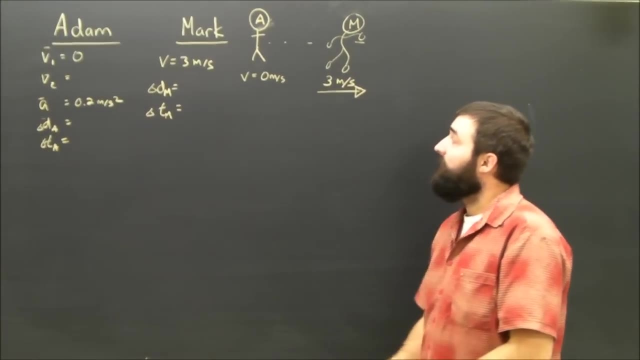 write dA and I'm going to write tA: the displacement of Adam and the time for Adam. The most common mistake for people who don't read the question very well and don't understand what they're doing is to go ahead and slap 30 meters as one of these distances And then they solve. 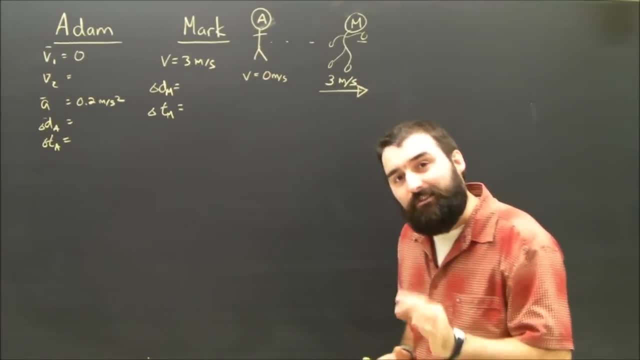 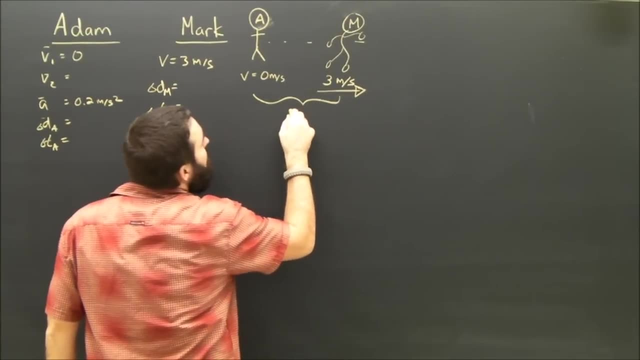 something and say: is this right? And it's, of course, totally wrong, Because look back at the question: What was 30 meters? 30 meters is the distance between the two of us, And the distance between the two of us is how far apart Adam and Mark are at the start, when t equals 0. Then at some point, 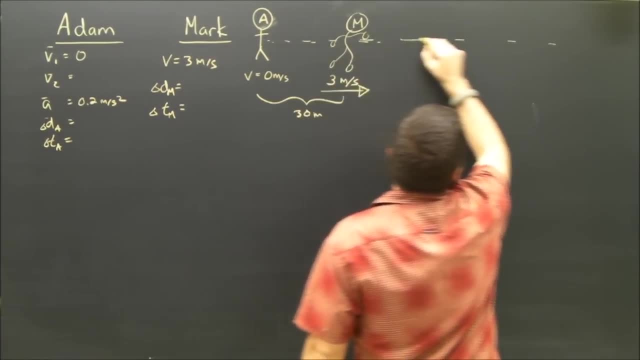 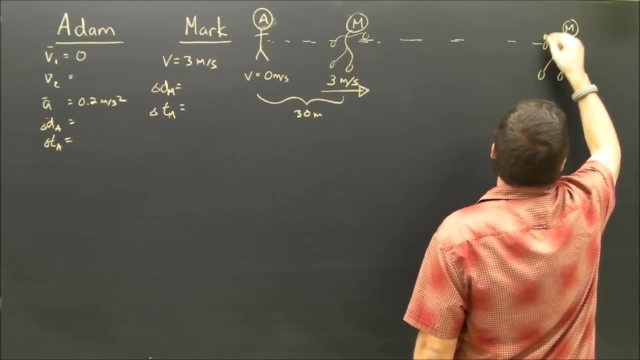 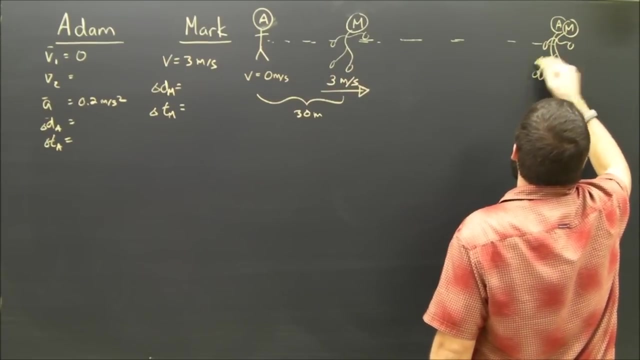 Mark is going to keep on running, But at some point Adam is going to speed up And eventually it won't take too long because Adam is much faster than Mark, But eventually they're going to be in the same place at the same time. 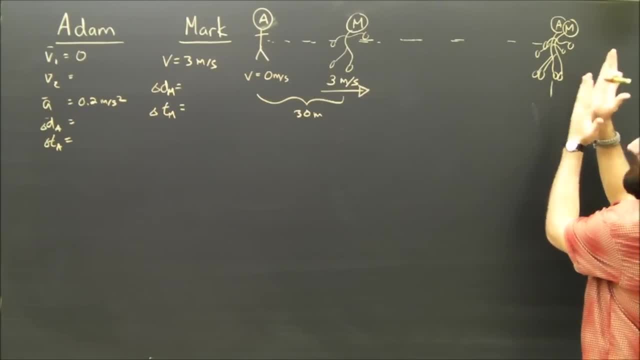 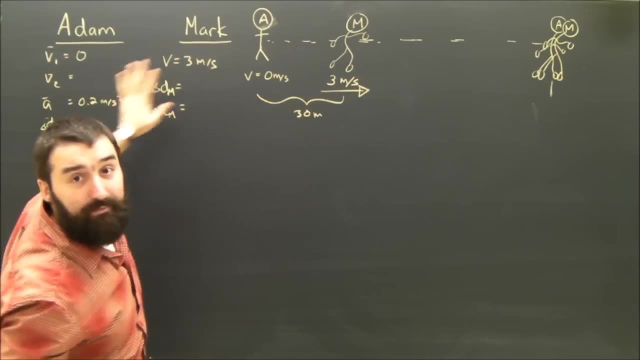 And that's the end of the race. Adam is now caught up to Mark. 30 meters was only the head start. That's not what d and the big five stand for. Delta d with the little arrow: It stands for displacement. how far they actually went. 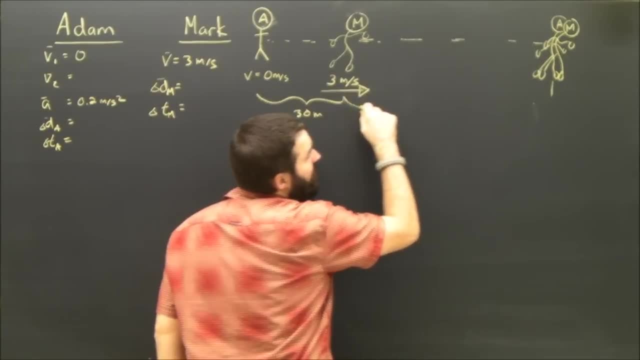 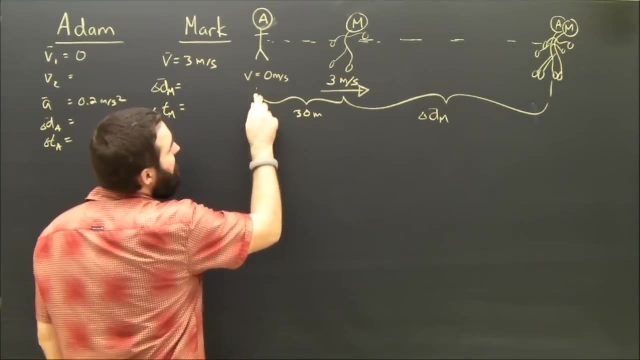 So how far did Mark actually go? for example, He started here and he ended up here. That is the displacement of Mark. What about Adam? Well, Adam started way over here And he ran 40 meters. When Mark turns around, he's replaced by a lower-ranked worker, If he's actually 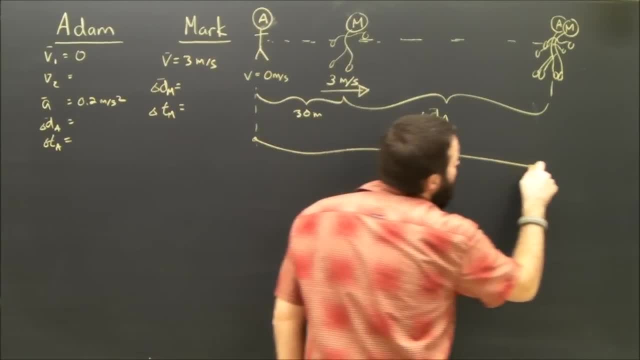 going to hit a 5-meter mark. he's going to hit a mentioning mark And that's the end of the race And the 30 meters. Andy ran as far as Mark had to run, so we're going to call that DA. 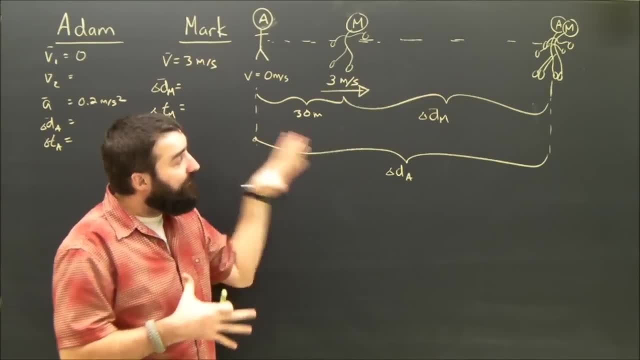 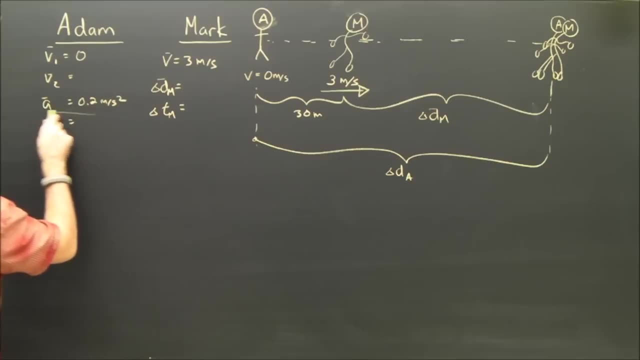 Now you can see the 30 meters. of course is part of the question, but it's not one of the gibbings. The question's a little harder than that. What is the question? The question was to find DA. What is the displacement of Adam? 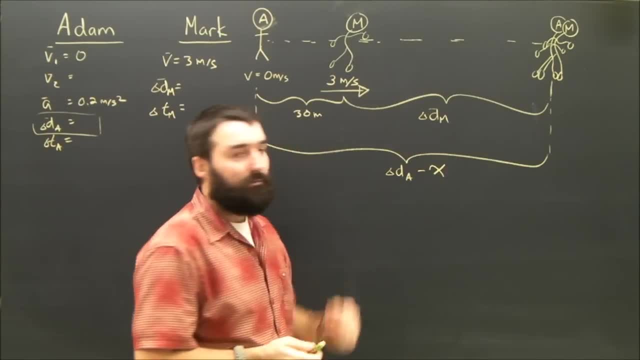 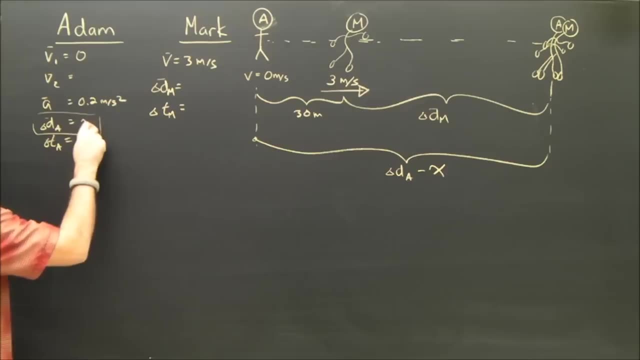 So I'm going to go ahead and I'm going to call that X. That's what we're trying to find. What is X? I'm going to call that X. so then over here I'm going to say X. Okay, if this is X and this is 30, then what's the displacement of Mark? 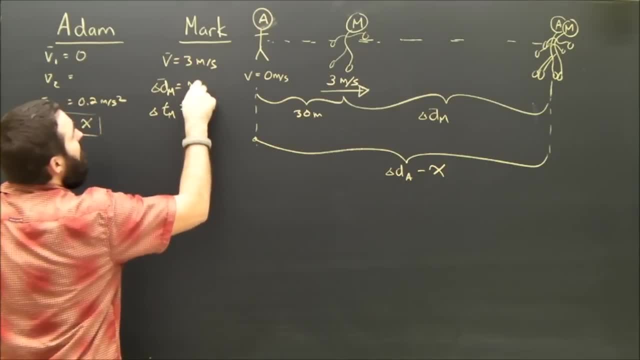 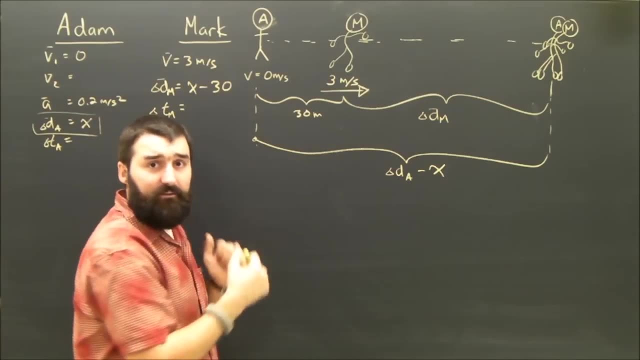 It's obviously X. take away 30.. X minus 30. And that takes care of the Ds. the only thing left is the time. But we started at zero and we caught up to them at a time of T, so the time for each of them is going to be T. 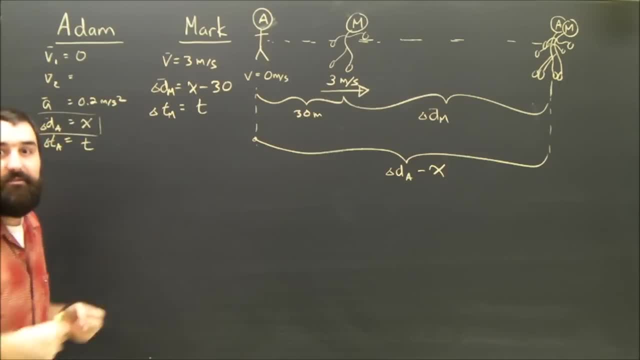 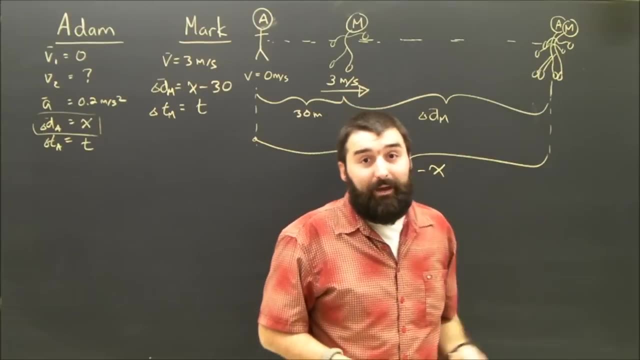 Again, I'm not really using those little question marks, because they don't matter. They don't help us figure out what formulas to use. I will use it, though, for V2, for Adam, because I don't care what Adam's velocity is when he passes Mark. 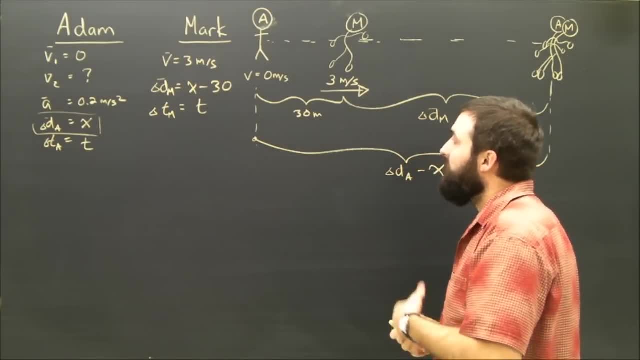 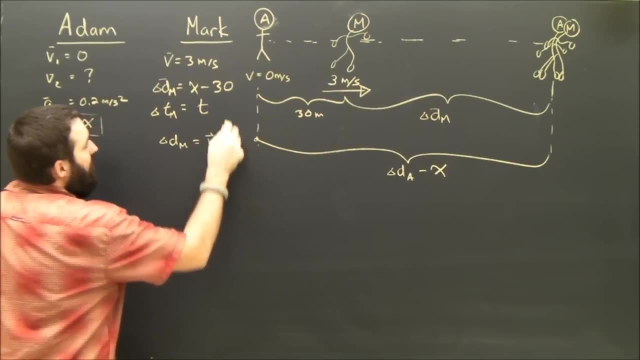 Although if this was a test I would probably make that part B of the question. So looking at Mark again, we see, we know that displacement equals velocity times time. Subbing in, we see that X minus 30 equals 3T. 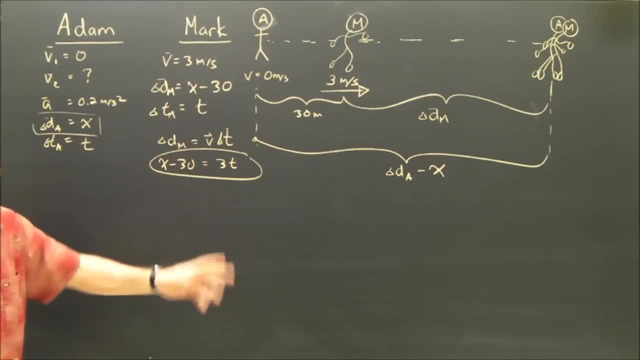 Again two equations. one equation, two unknowns. We can't solve that. We need another equation here. Looking at Adam, we see that D equals V1T plus a half AT squared. Subbing in again, V1 is zero disappears. that's convenient. 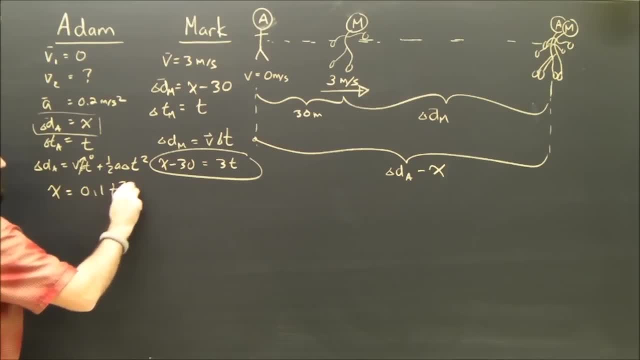 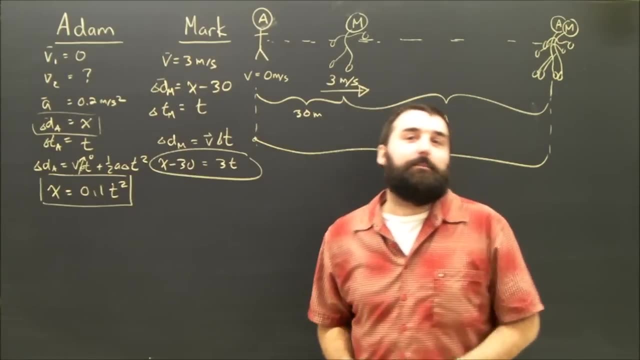 We see that X equals 0.1T squared, And I have taken a shortcut. I have not followed my own advice. I didn't show the substitution, I skipped a step. Hopefully I didn't make a mistake Putting the two equations together. 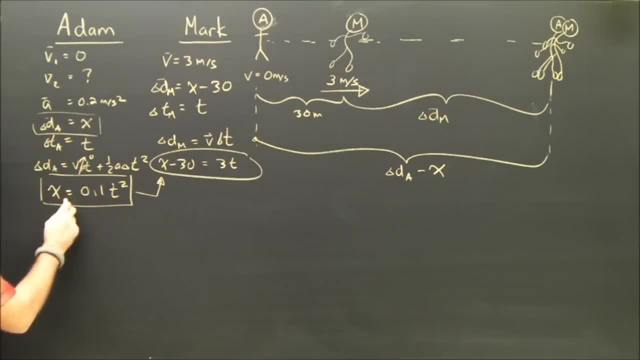 if I sub this equation into that equation, I will get that 0.1T squared minus 30 equals 3T. Rearranging this because it is of course a quadratic equation, I get that. I like to use my not super smart calculator, but pretty smart. 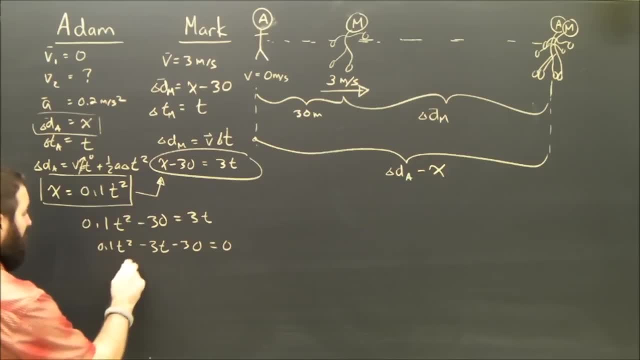 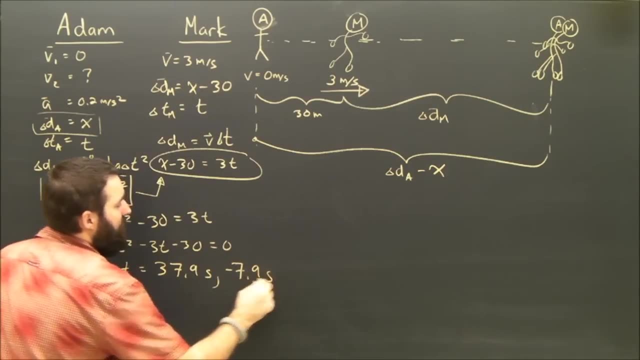 it's not a graphic calculator to answer that. It doesn't take very long and I see quadratic formula that T is either 37.9 seconds or negative 7.9 seconds. Subtitles by the Amaraorg community. Subtitles by the Amaraorg community. 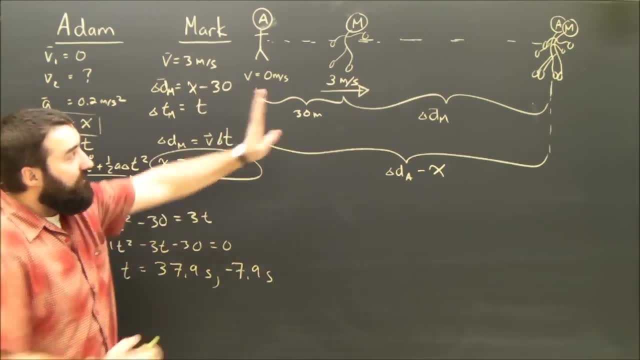 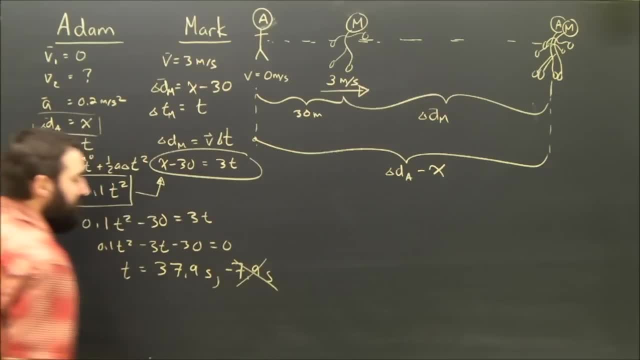 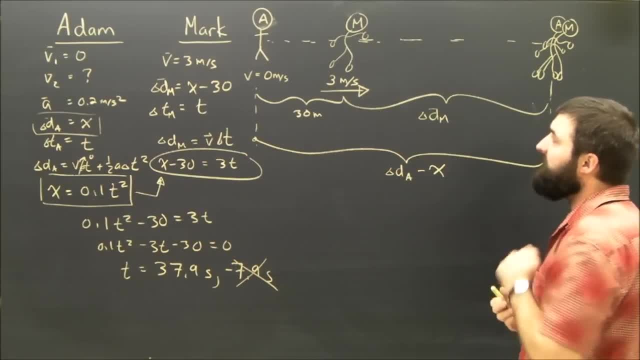 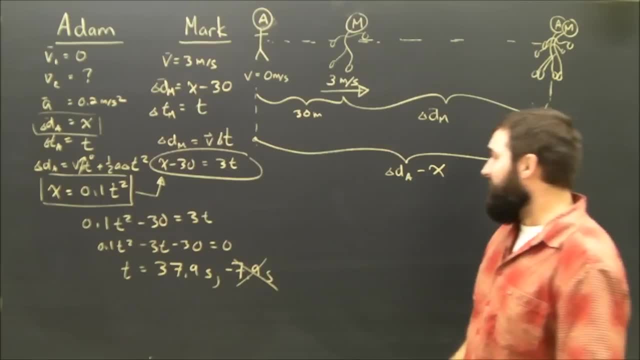 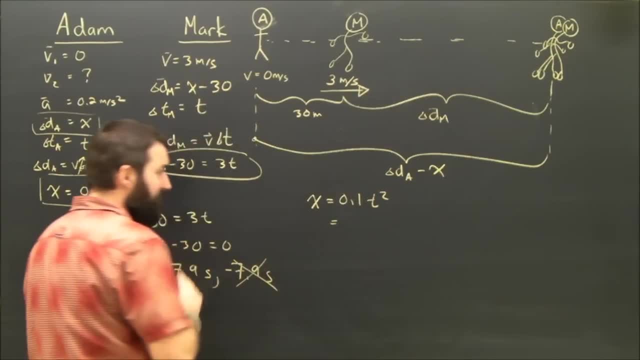 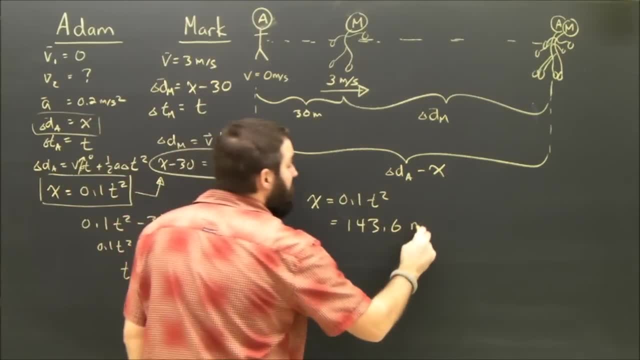 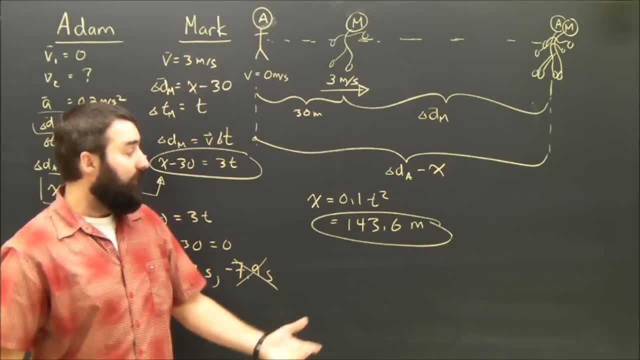